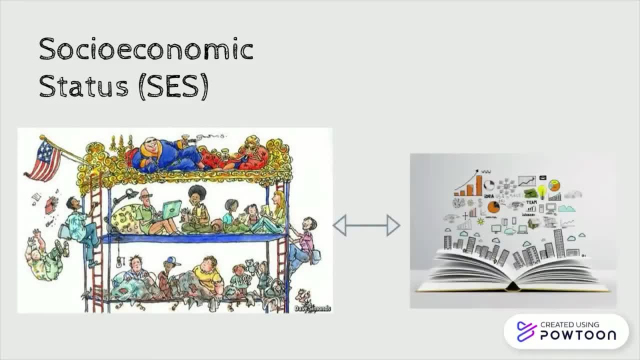 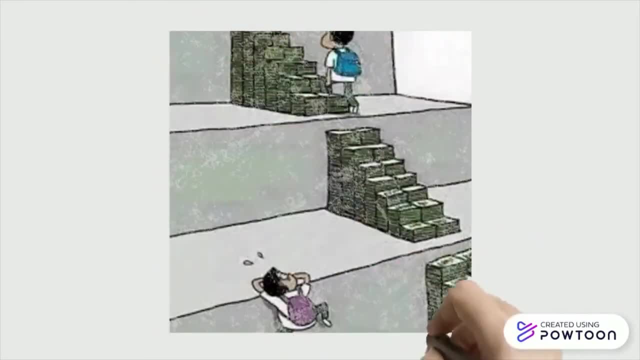 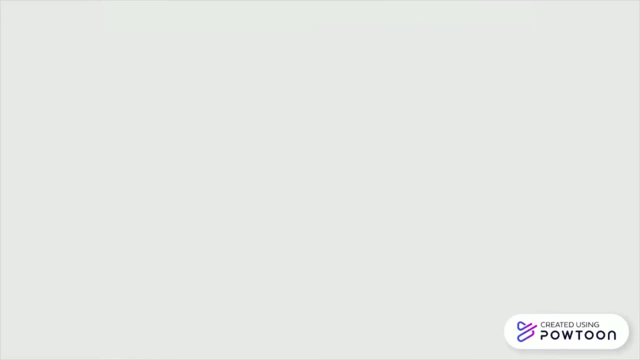 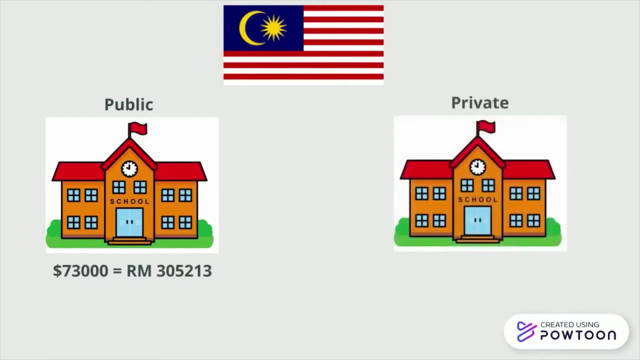 This is increasingly relevant in the educational society today, as a low SES has been linked to poorer educational achievement. Education inequality can be linked to students' family background. Many believe that private education is the root cause of education inequality. For example, the cost of public school in Malaysia is $73,000 from preschool to year 12, while the cost of private school is $1 million. 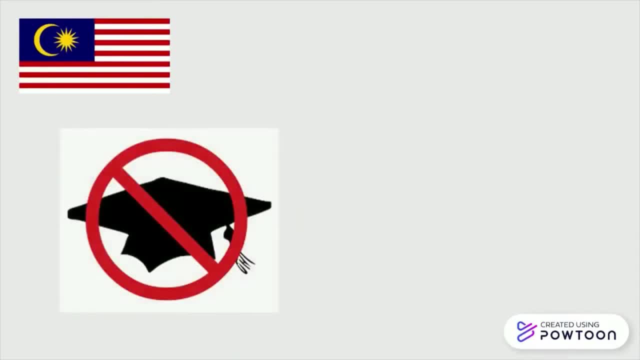 Referring to Malaysia, students who dropped out of secondary school before SPM mostly came from low-income groups. In 2014,, 42.12% dropped out of school at Form 1 due to poverty, learning difficulties and underage marriage. 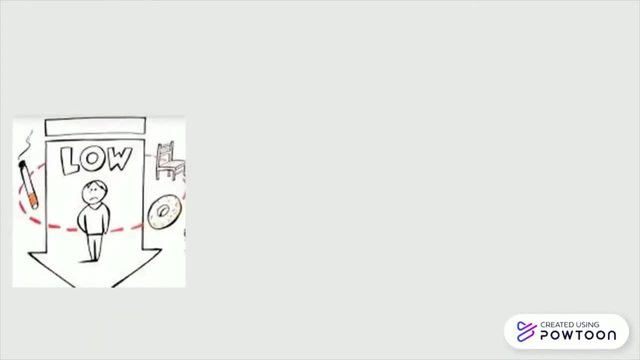 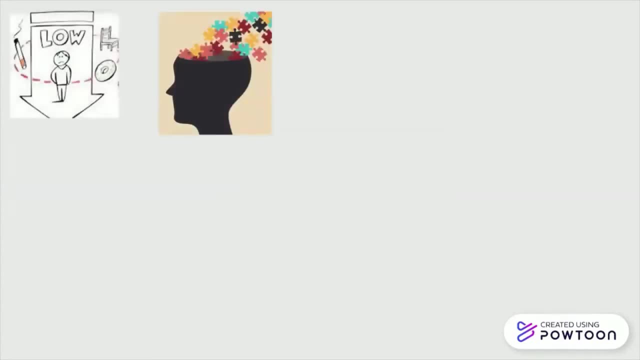 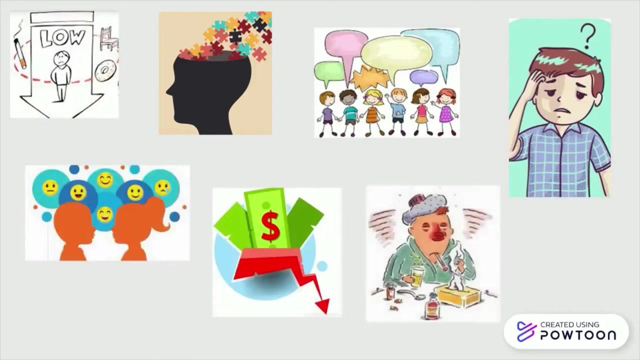 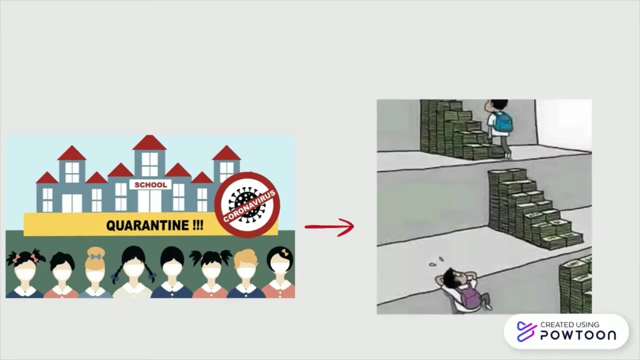 Research also shows that children of low SES households develop academic skills slower than those from high SES status, As related to poor cognitive development, language, memory, socio-emotional processing and, consequently, poor income and health in adulthood. Furthermore, the COVID-19 pandemic has also caused education inequality by widening the education gap between advanced economies and middle- and low-income nations unable to provide online learning. 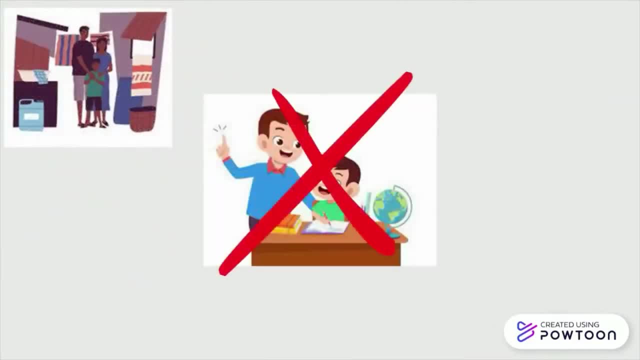 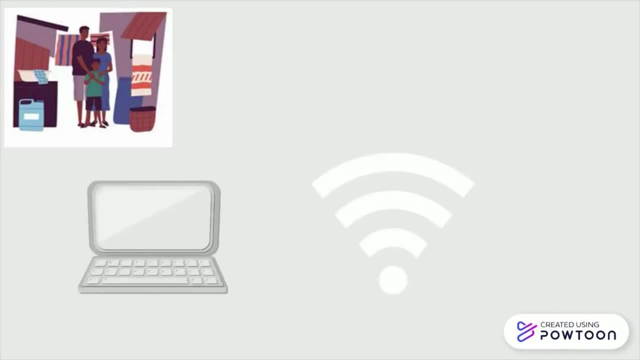 Low-income parents are unable to support their child's learning from home due to the need of technology like laptops or the internet. In addition, even if parents were able to provide the technology, low-SES kids are more likely to have unreliable internet access. 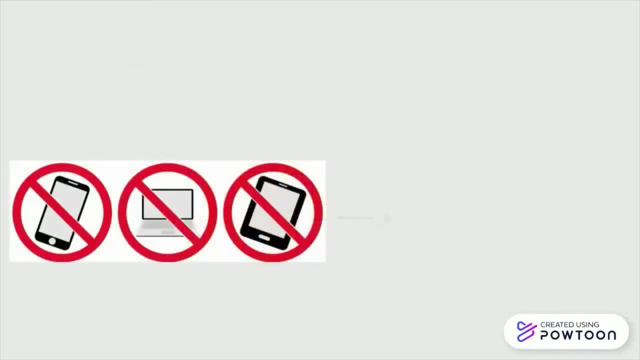 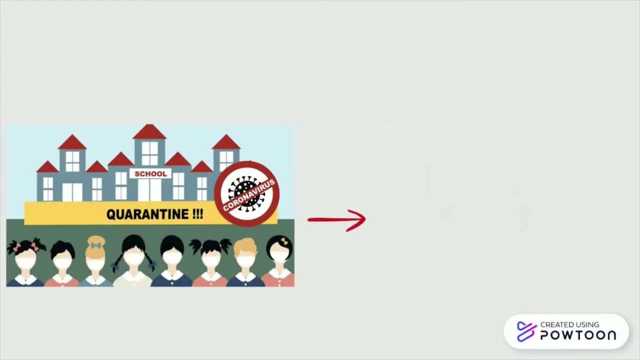 The school systems in low-SES communities are often under-resourced, negatively affecting students' academic progress. Moreover, the current COVID crisis may result in a greater impact on the socio-economic status of education as budgets fall more quickly as public revenues decline sharply. 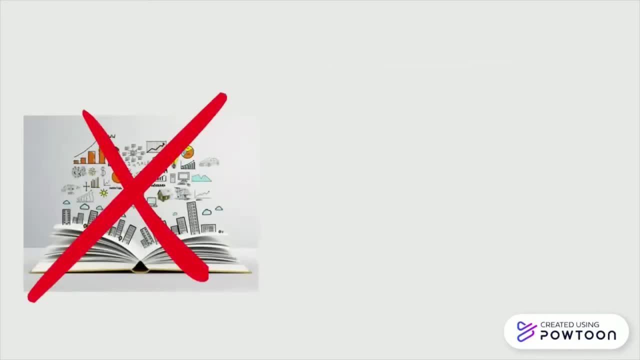 The governments may find it difficult to fund for education, as the spending has to be prioritised more on health. Therefore, low-income households may not be able to afford to support their child's learning. Therefore, low-income households may not be able to support their child's learning. 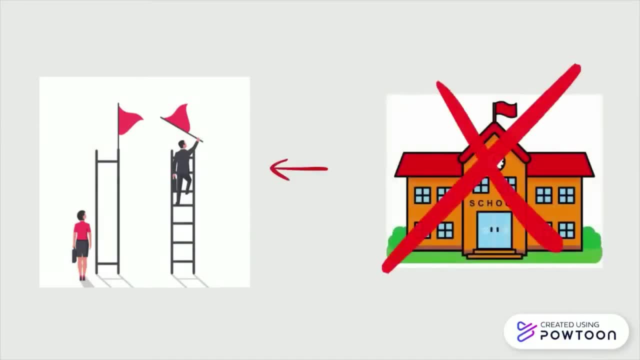 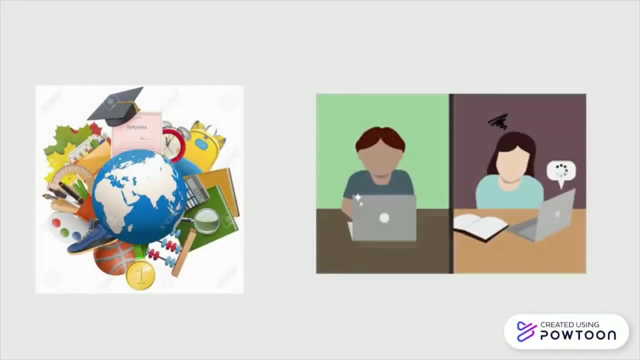 Therefore, low-income households may not be able to support their child's learning. This may be a disadvantage, since they are unable to spend on private woes. However, many educational systems across the globe are finding methods to respond to the challenges of online learning of for lower-SES children.